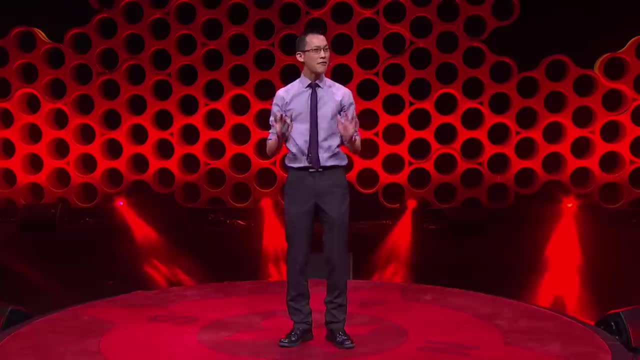 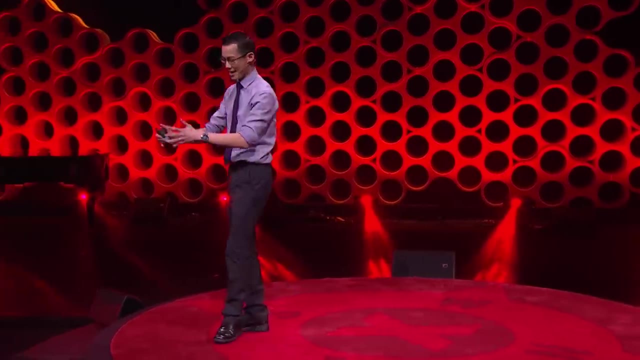 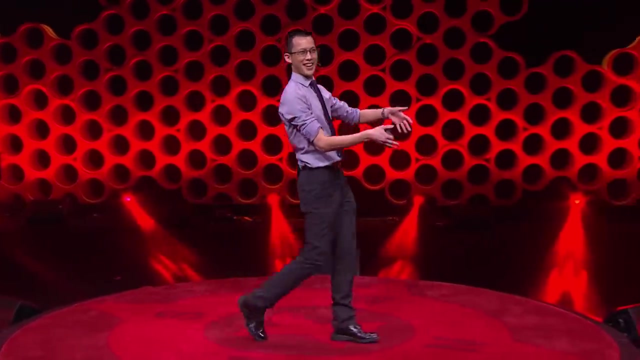 Australian mathematics competition and we'd print out a list of everyone in the class, the school, in order of our scores. Students who received prizes and high distinctions were pinned up at the start of a long corridor, far, far away from the dark and shameful place where my name appeared. 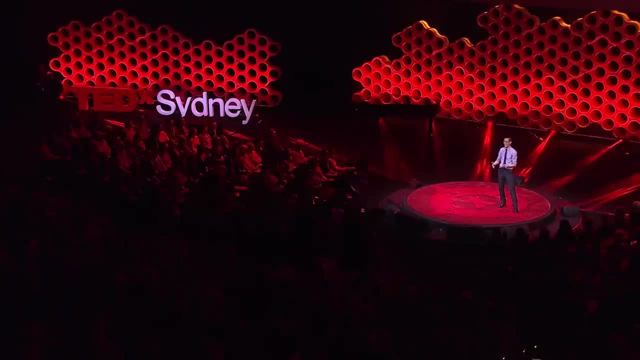 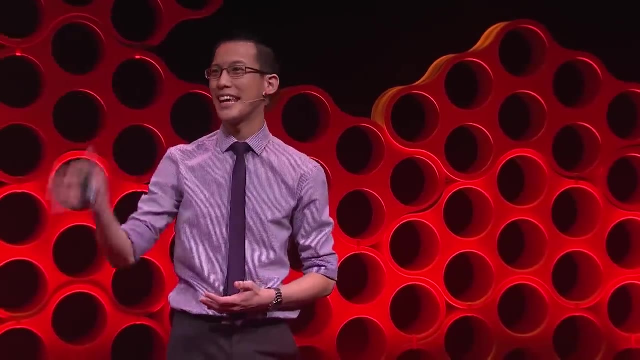 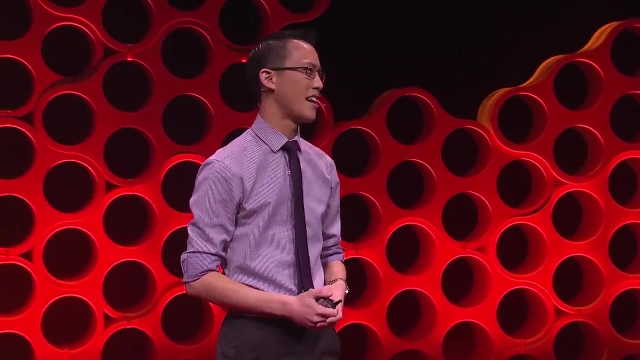 Maths was not really my thing. Stories, characters, narratives- this is where I was at home And that's why I raised my sales and set course to become an English and history teacher. But a chance encounter at senior university altered my life forever. 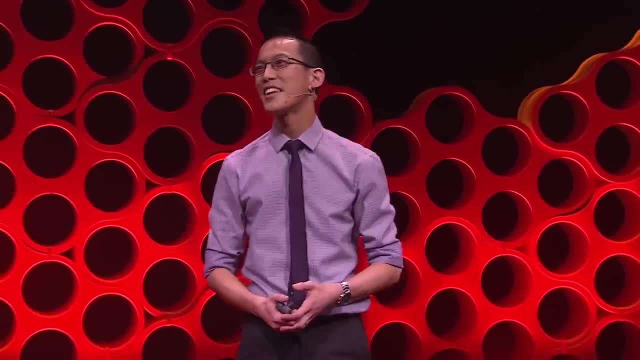 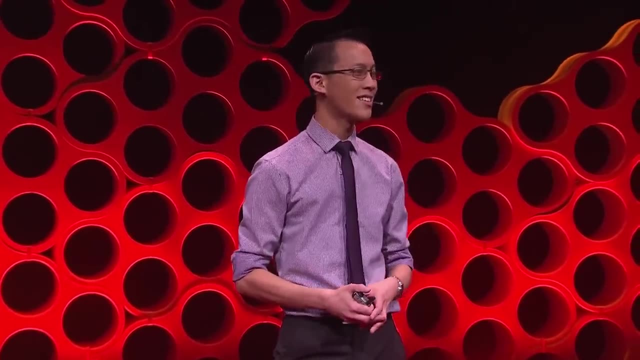 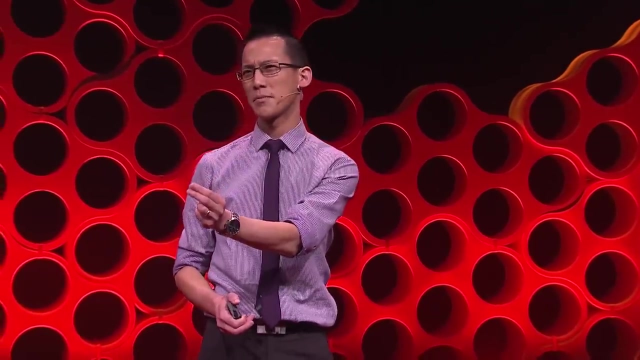 I was in line to enroll at the faculty of education when I started a conversation with one of its professors. He noticed that, while my academic life had been dominated by humanities, I had actually attempted some high level maths at school, And what he saw was not that I had a problem with maths, but that I had perceived it as a problem. He noticed that, while my academic life had been dominated by humanities, I had actually attempted some high level maths at school. He noticed that, while my academic life had been dominated by humanities, I had actually persevered with maths. 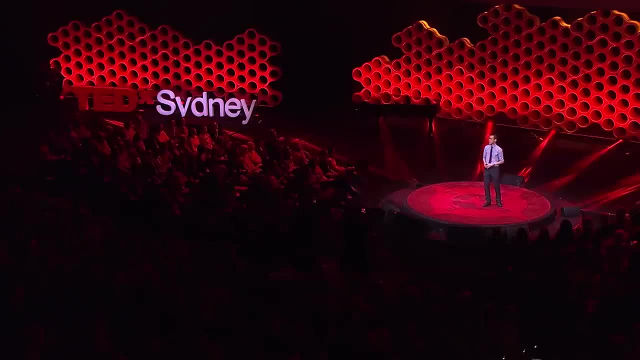 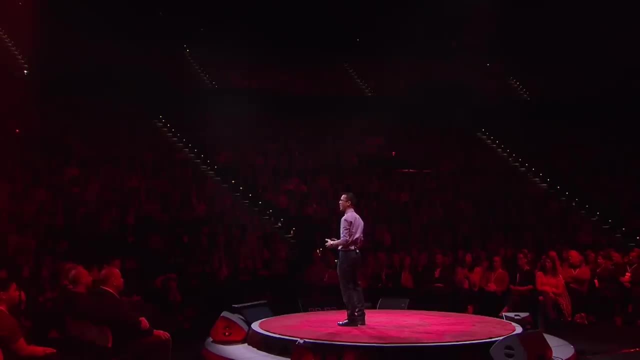 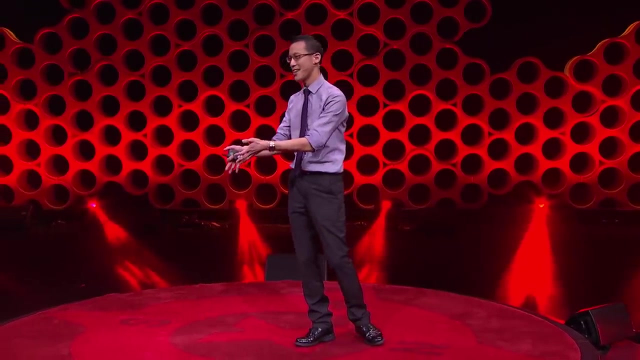 And he knew something I didn't: that there was a critical shortage of mathematics educators in Australian schools, a shortage that remains to this day. So he encouraged me to change my teaching area to mathematics. Now, for me, becoming a teacher wasn't about my love for a particular subject. 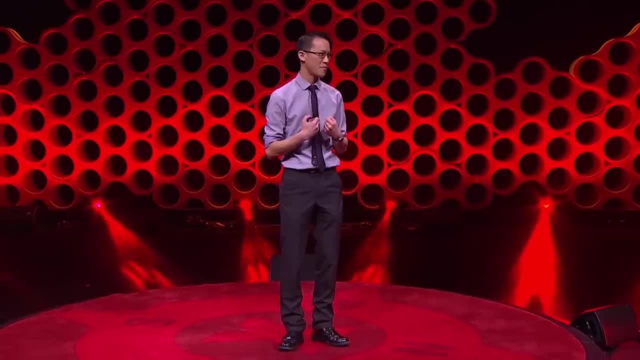 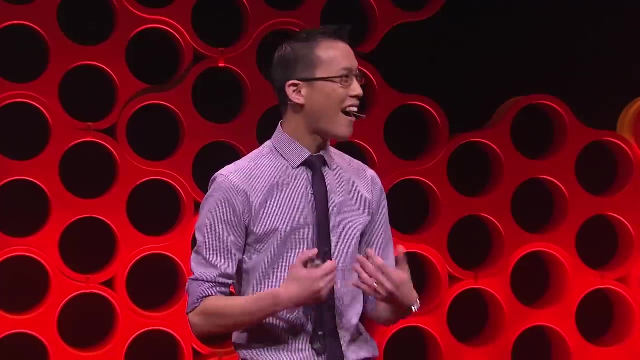 It was about having a personal impact on the lives of young people. I'd seen firsthand at school what a lasting and positive difference a great teacher can make. I wanted to do that for someone, and it didn't matter to me what subject I did it in. 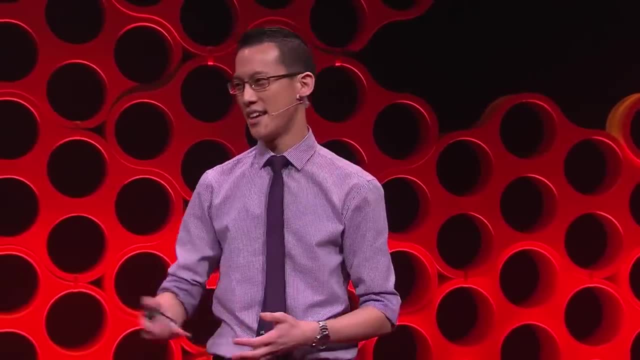 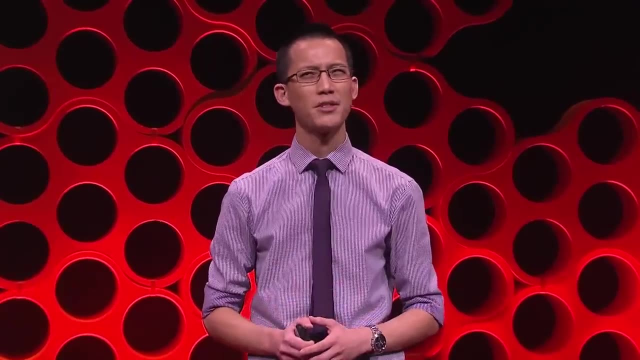 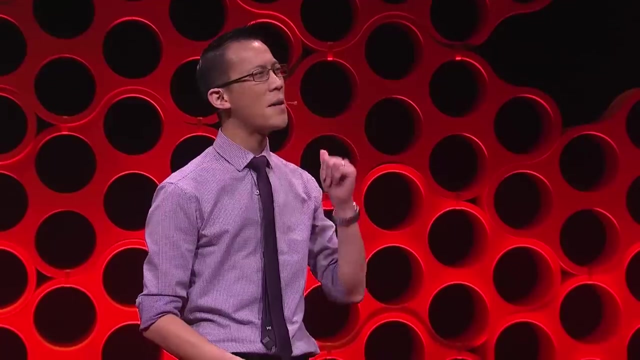 If there was an acute need in mathematics, then it made sense for me to go there. As I studied my degree, though, I discovered that mathematics was a very different subject to what I'd originally thought. I'd made the same mistake about mathematics that I'd made earlier in my life about music. 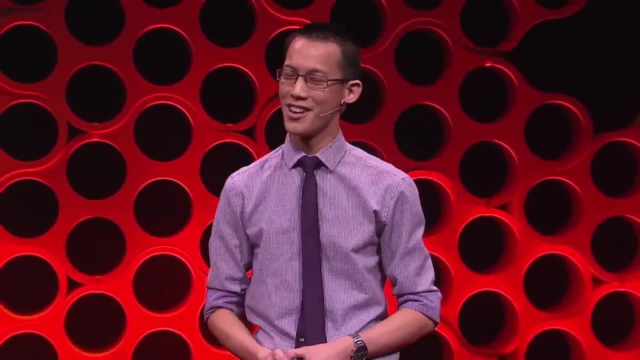 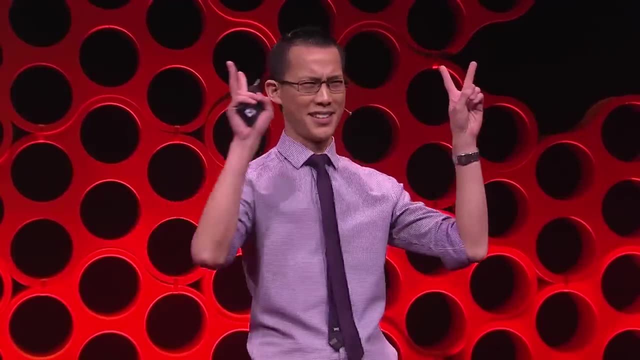 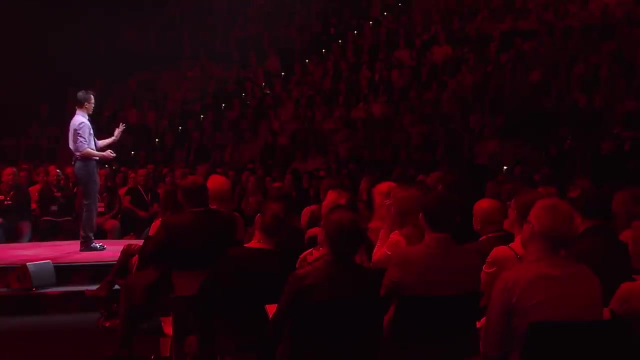 Like a good migrant child, I dutifully learned to play the piano when I was young. My weekends were filled with endlessly repeating scales and memorizing every note in the piece Spring and Winter. I lasted two years before my career was abruptly ended when my teacher told my parents his 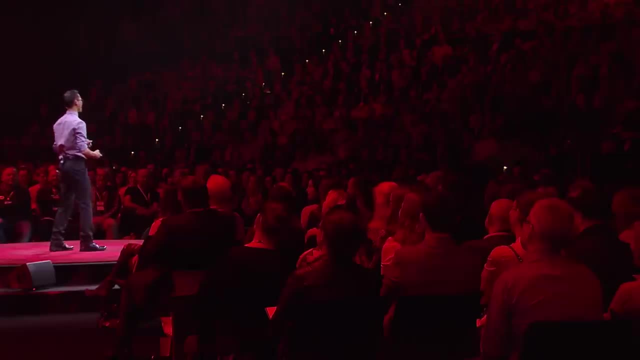 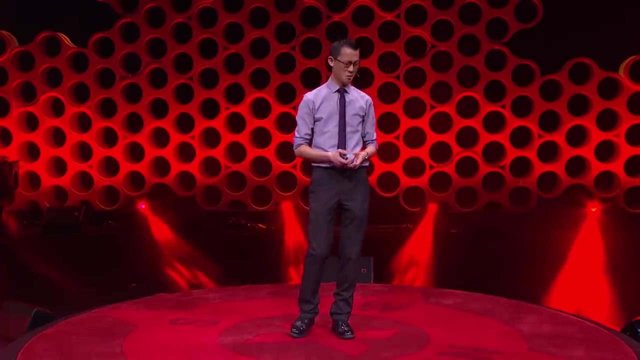 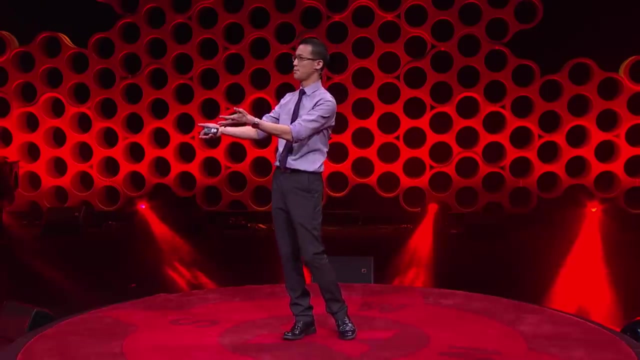 fingers are too short. I will not teach him any more. At seven years old, I thought of music like torture. It was a dry, solitary, joyless exercise that I only engaged with because someone else perhaps forced me to. It took me 11 years to emerge from that sad place. 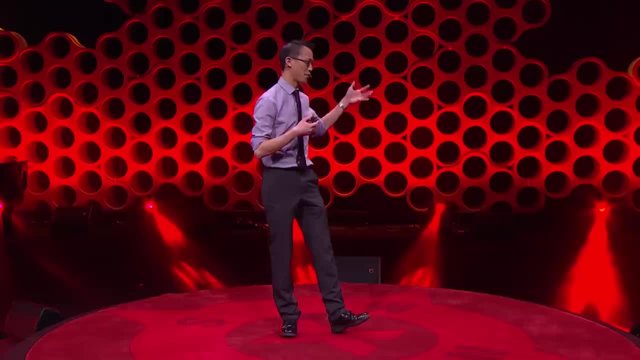 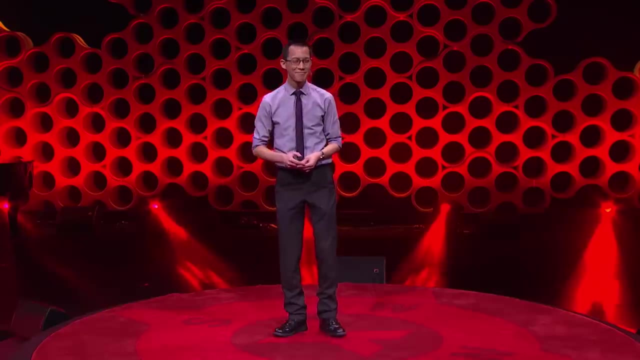 In year 12, I picked up a steel string acoustic guitar for the first time. I wanted to play it for church, and there was also a girl I was fairly keen on impressing, so I convinced my brother to teach me a few chords. 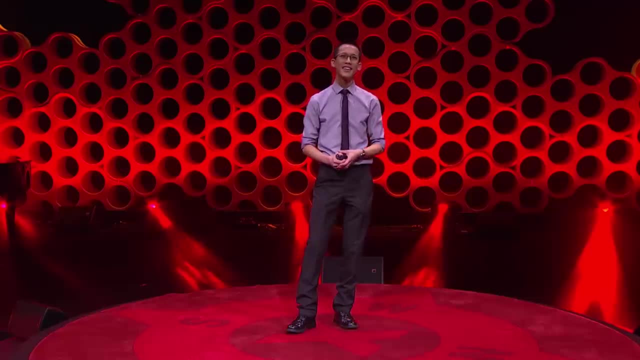 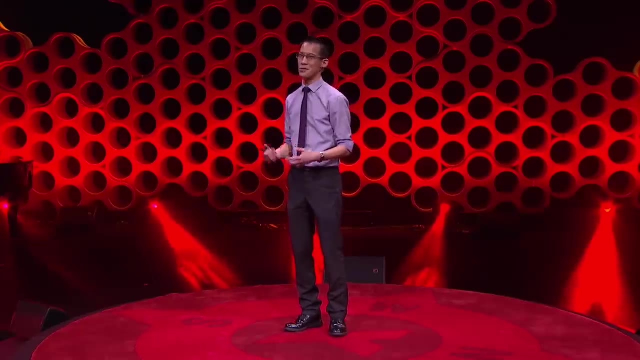 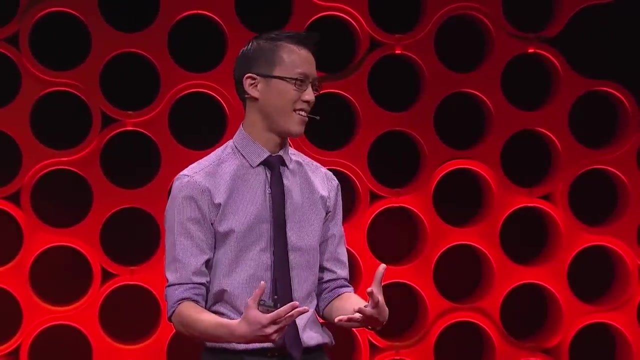 And slowly but surely, my mind changed. I was engaged in a creative process. I was making music And I was hooked. I started playing in a band and I felt the delight of rhythm pulsing through my body as we brought our sounds together. 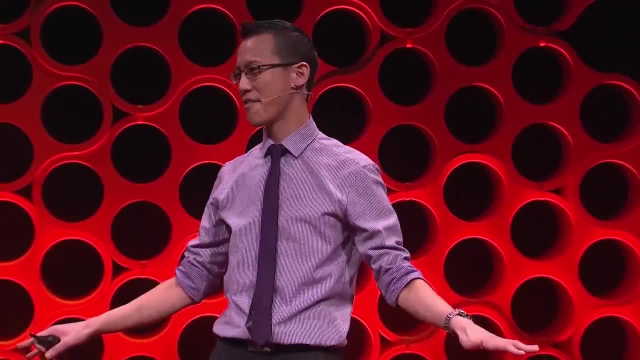 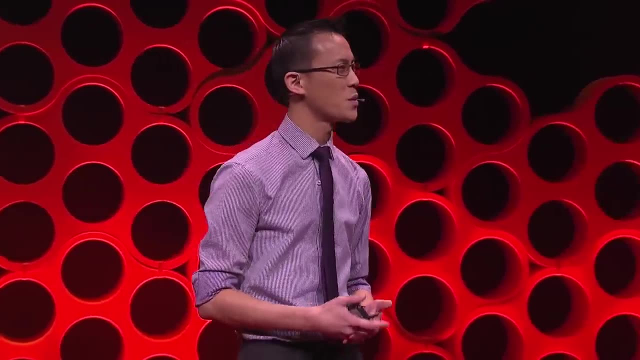 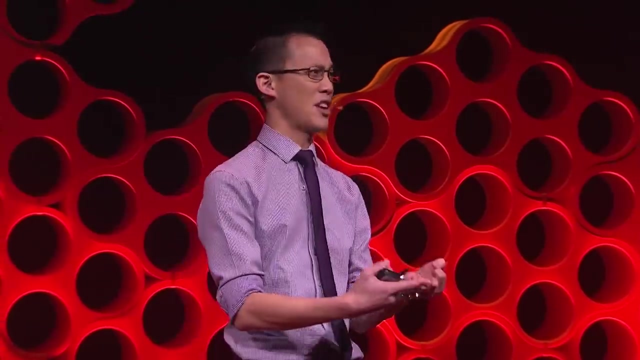 I'd been surrounded by a musical ocean my entire life and for the first time I realized I could swim in it. I went through an almost identical experience when it came to mathematics. I used to believe that maths was about rote learning and scrutable formulas to solve abstract. 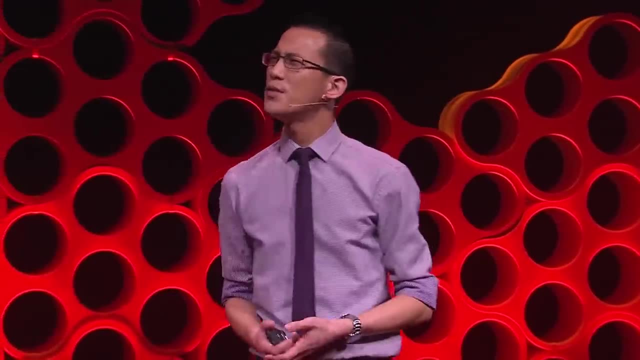 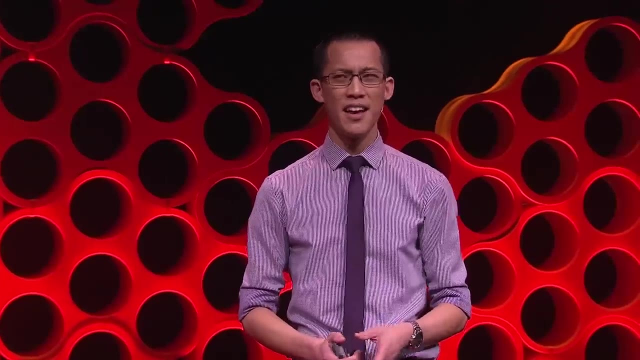 problems. that didn't mean anything to me, But it used to be that I was a genius. But at university I began to see that mathematics is immensely practical and even beautiful, That it's not just about finding answers but also about learning to ask the right questions. 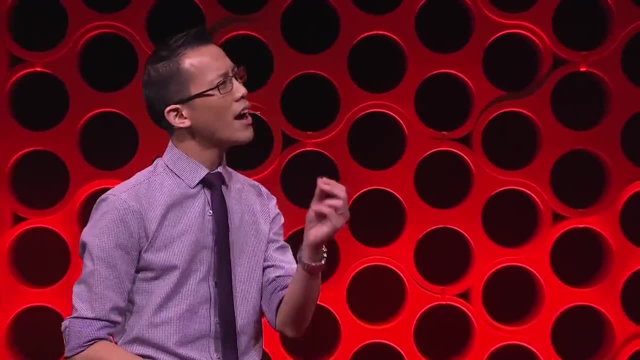 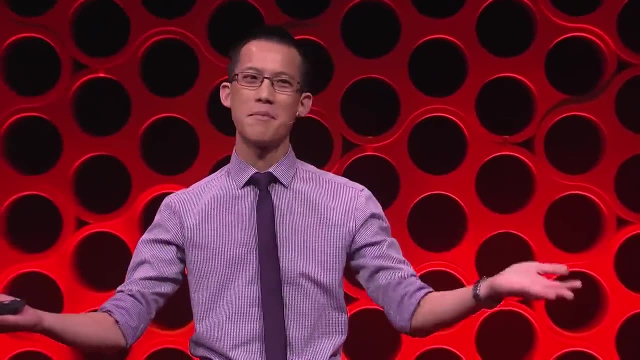 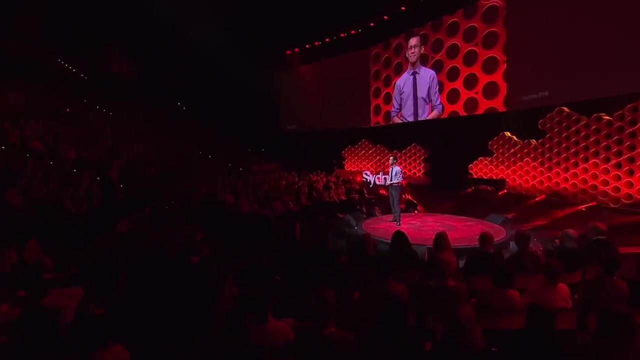 And that mathematics isn't about mindlessly crunching numbers, but rather about forming new ways to see problems so we can solve them. by combining insight with imagination, It gradually dawned on me. It dawned on me That mathematics is a sense. 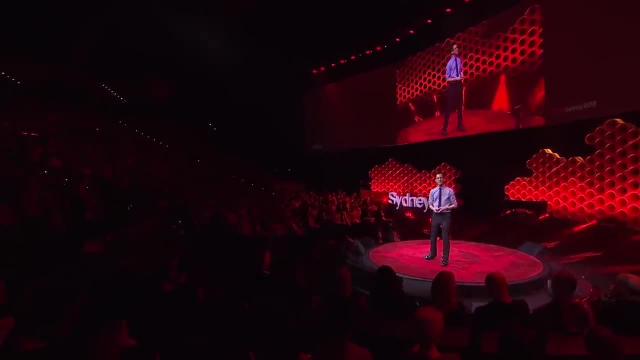 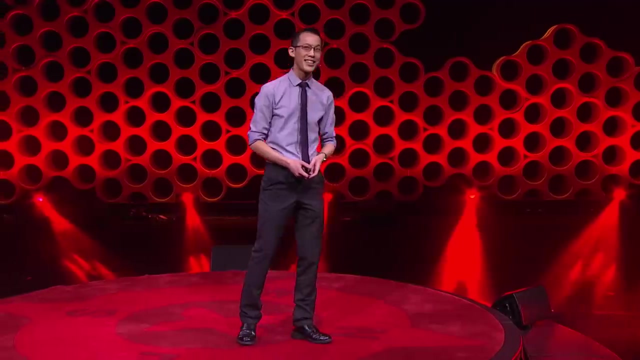 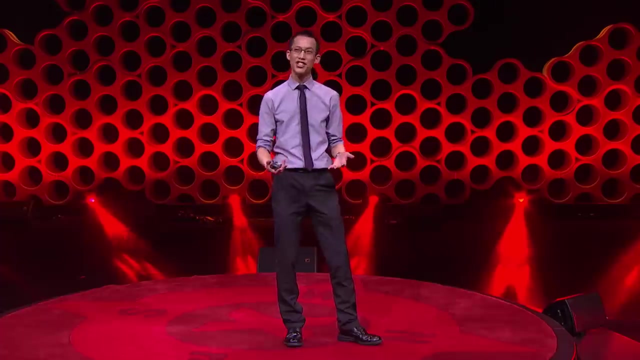 Mathematics is a sense, just like sight and touch. It's a sense that allows us to perceive realities which would be otherwise intangible to us. You know, we talk about a sense of humor and a sense of rhythm. Mathematics is our sense for patterns, relationships and logical connections. 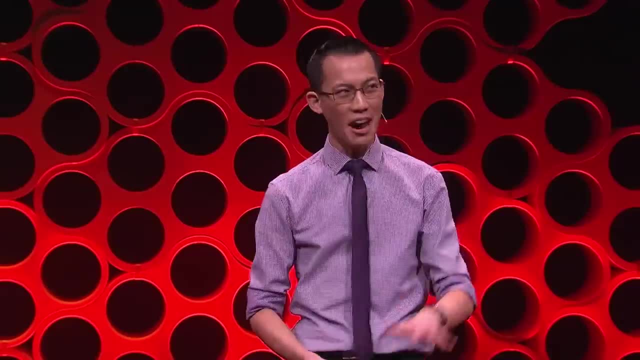 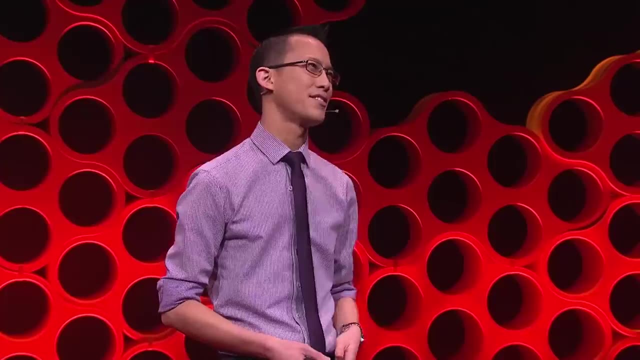 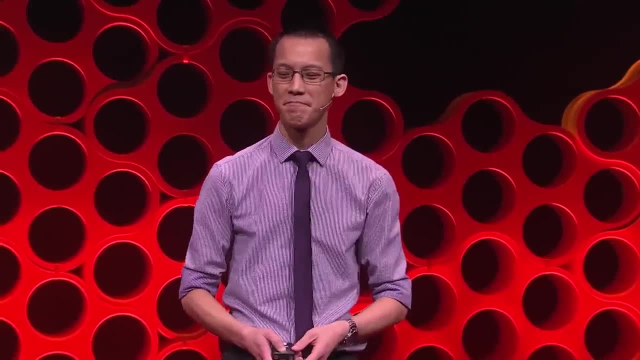 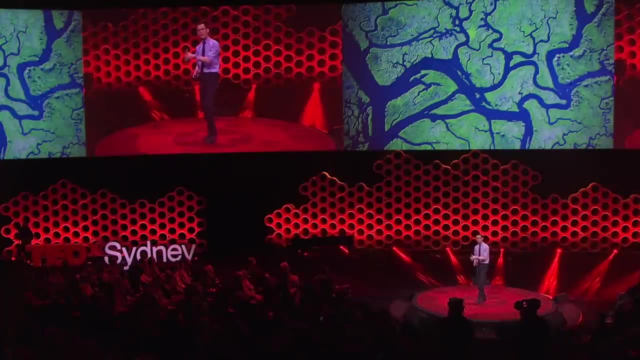 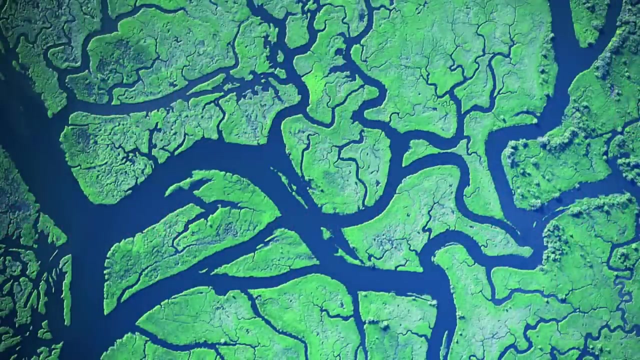 It's been hidden in plain sight your entire life. This is a river delta. It's a beautiful piece of geometry. Now, when we hear the word geometry, most of us think of triangles and circles, But geometry is the mathematics of all shapes and this meeting of land and sea has created. 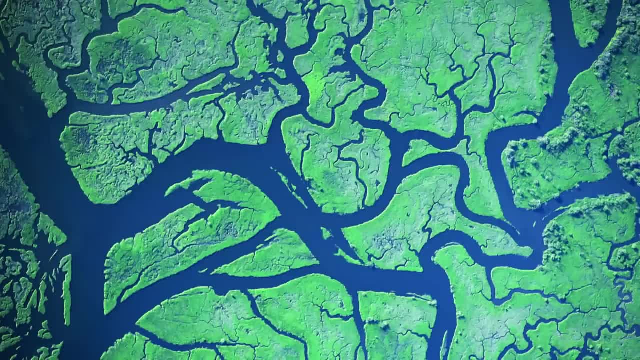 shapes with an undeniable pattern. It has a mathematically recurrent pattern. It has a mathematically recurrent pattern And it's a recursive structure. Every part of the river delta, with its twists and turns, is a microversion of the greater. 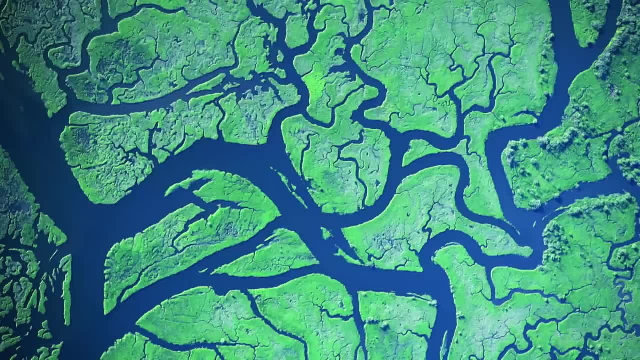 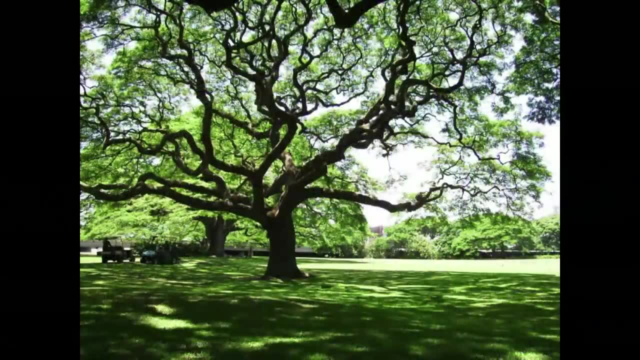 whole. I want you to see the mathematics in this, But that's not all. I want you to compare this river delta with this amazing tree. It's a wonder in itself, but focus with me on the similarities between this and the river. 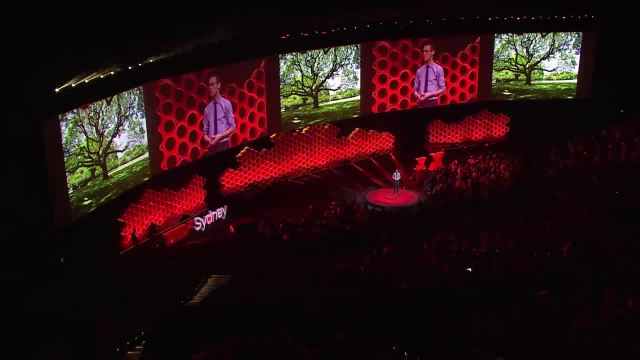 What I want to know is: why on earth are we talking about these things? Why on earth should these shapes look so remarkably alike? Why should they have anything in common? Things get even more perplexing when you realize it's not just water systems and plants that 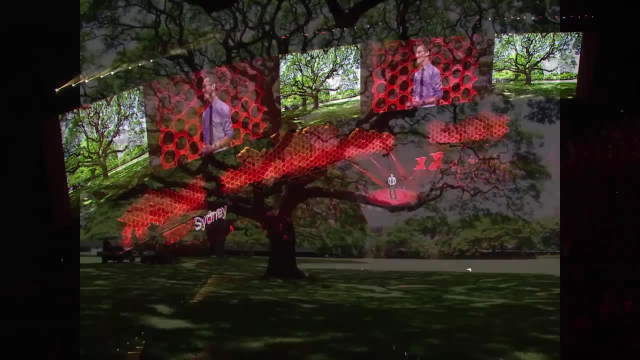 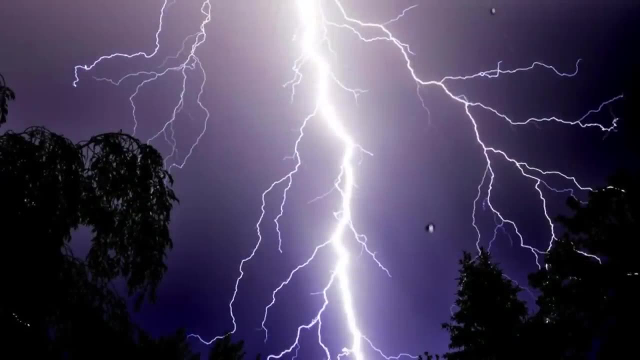 do this. If you keep your eyes open, you'll see. these same shapes are everywhere. Lightning bolts disappear so quickly that we seldom have the opportunity to ponder their geometry, But their shape is so unmistakable and so similar to what we've just seen that one can't. 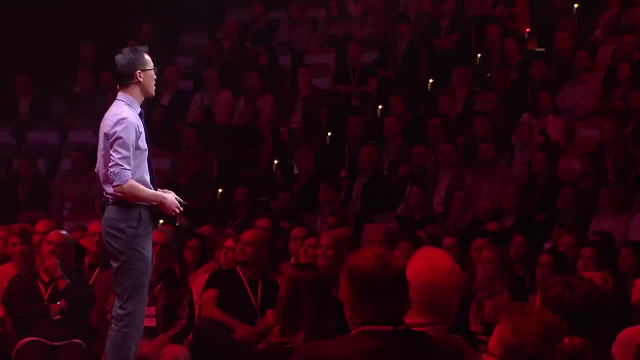 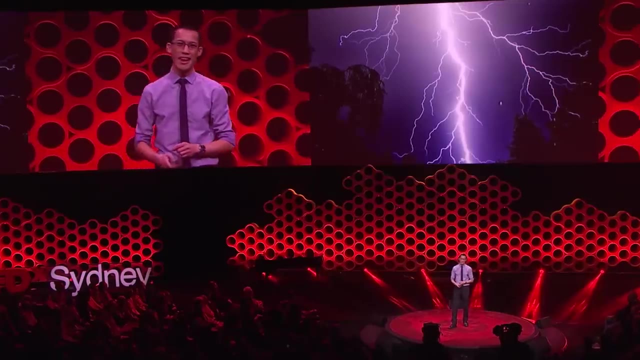 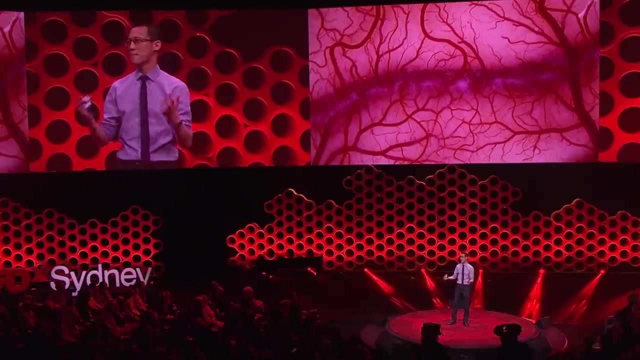 help but be suspicious. And then there's the fact that every single person in this room is filled with these shapes too. Every cubic centimeter of your body is packed with blood vessels that trace out this same pattern. There's a mathematical reality woven into the fabric of the universe that you share. 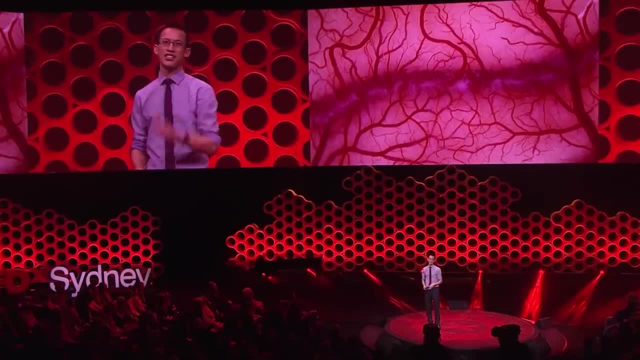 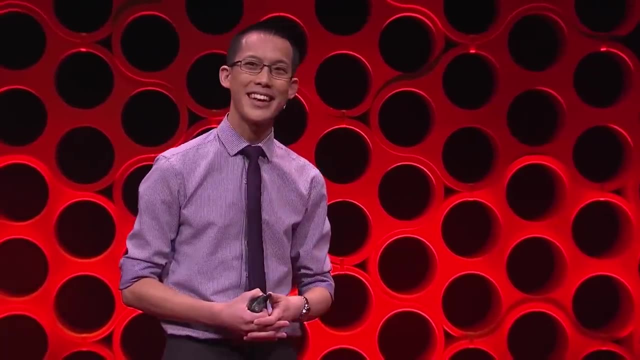 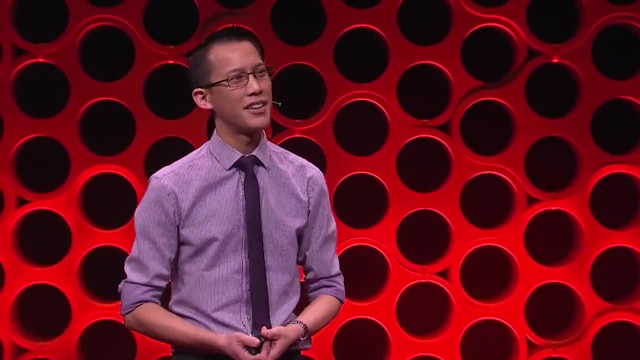 with winding rivers, towering trees and raging storms. These shapes are examples of what we've seen. They're what we call fractals. as mathematicians, Fractals get their name from the same place as fractions and fractures. It's a reference to the broken and shattered shapes we find around us in nature. 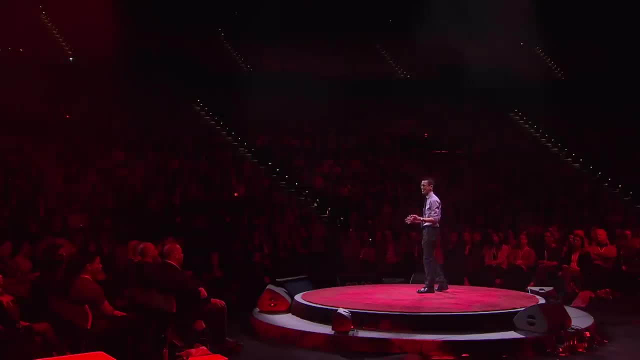 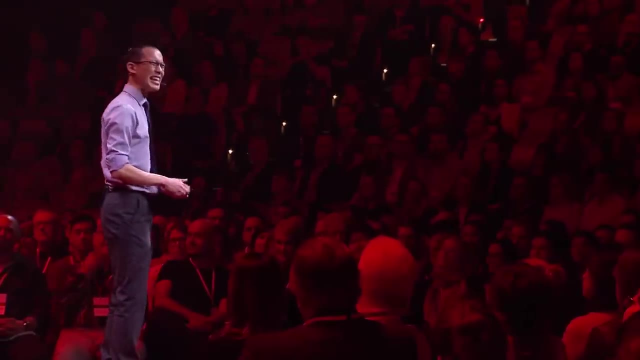 Now, once you have a sense for fractals, you really do start to see them everywhere, Ahead of broccoli, the leaves of a fern, even clouds in the sky. Like the other senses, our mathematical sense can be refined with practice. Where are all these things? practice. It's just like developing perfect pitch or a taste for wines. You can learn to perceive the mathematics around you with time and the right guidance. Naturally, some people are born with sharper senses than the rest of us. Others are born with impairment. 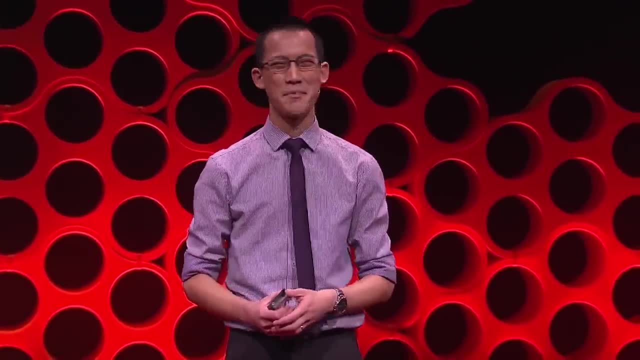 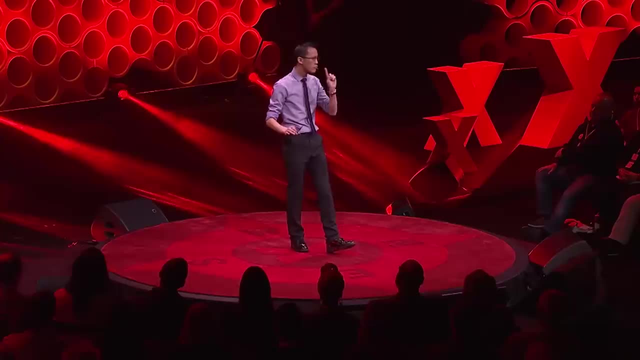 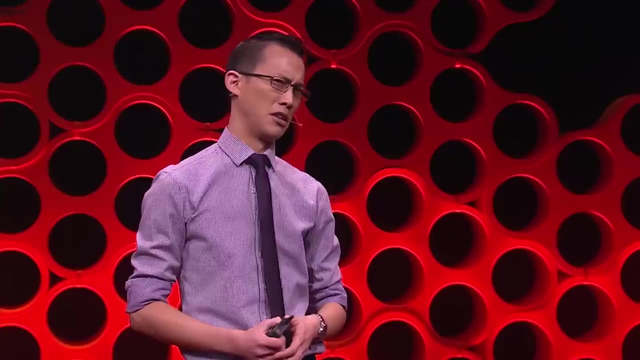 As you can see, I drew a short straw in the genetic lottery when it came to my eyesight. Without my glasses, everything is a blur. I've wrestled with this sense my entire life, but I would never dream of saying well, seeing has always been a struggle for me, I guess. 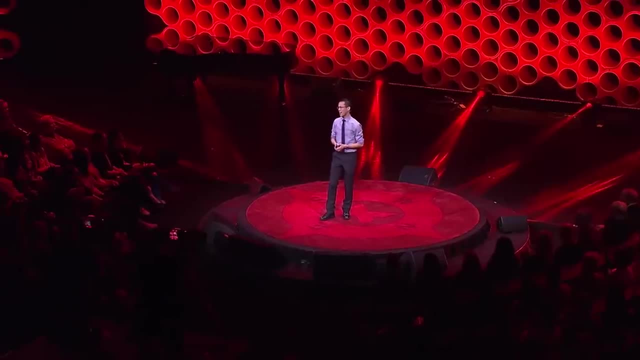 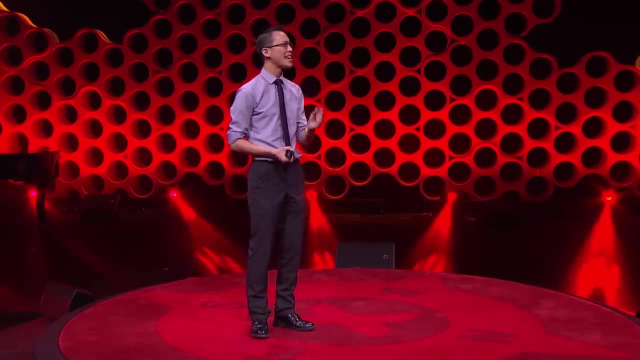 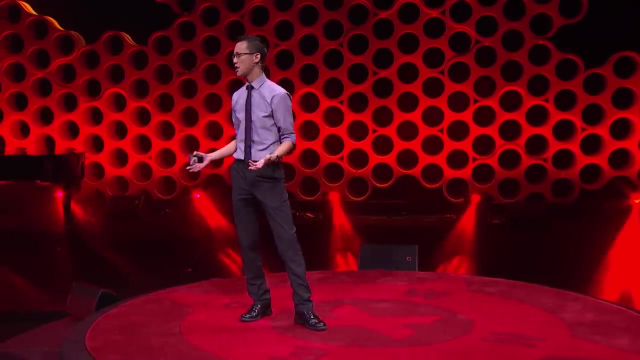 I'm just not a seeing kind of person. Yet I meet people every day who feel it quite natural to say exactly that about mathematics. I'm convinced we close ourselves off from a huge gap. It's a huge part of the human experience if we do this, because all human beings are. 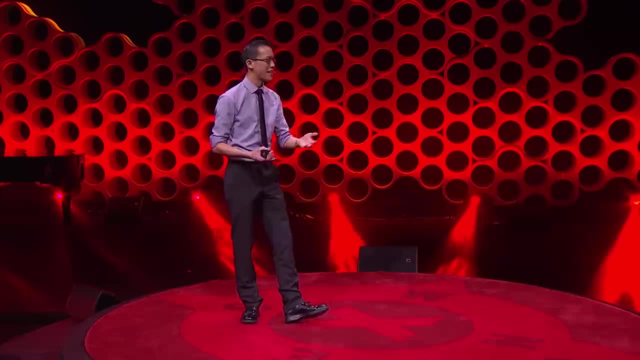 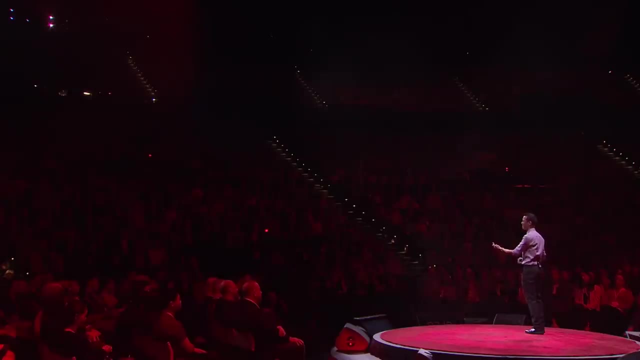 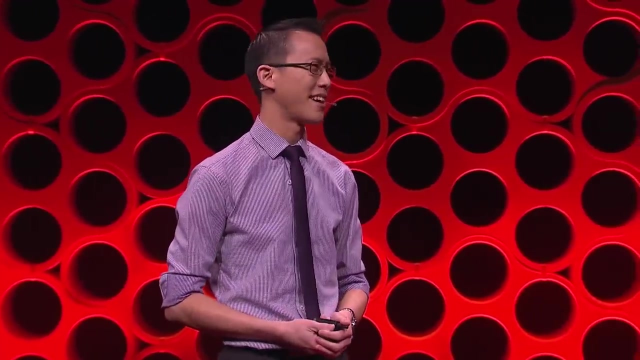 wired to see patterns. We live in a patterned universe, a cosmos. That's what cosmos means: orderly and patterned, as opposed to chaos, which means disorderly and random. It isn't just seeing patterns that humans are so good at. We love making patterns too. The people 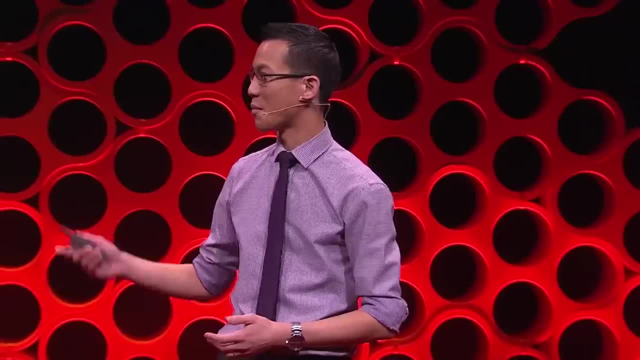 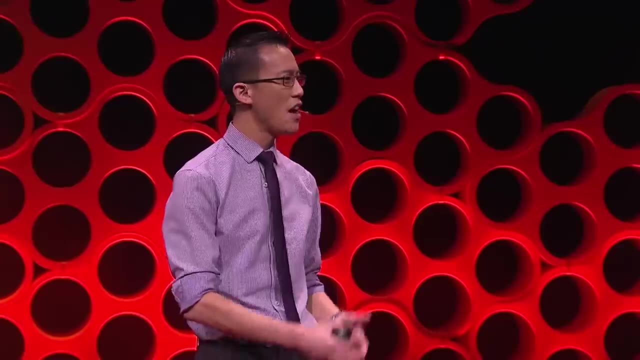 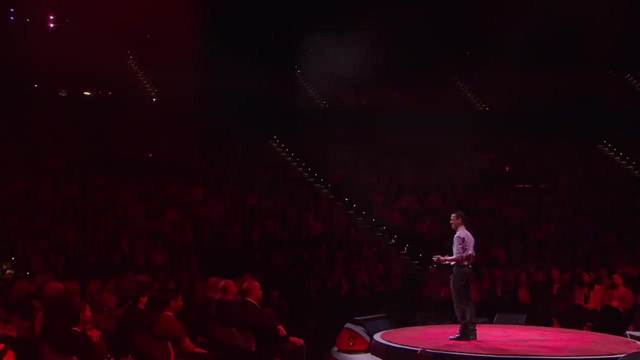 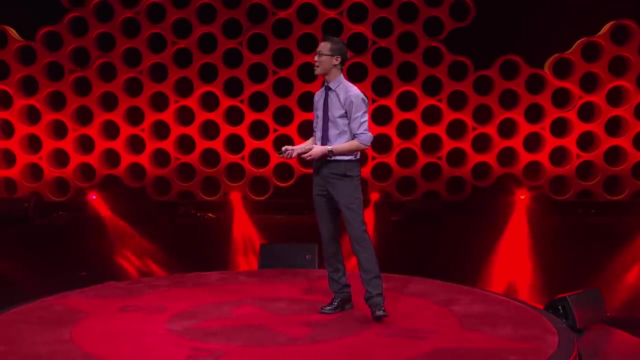 who do this well have a special name. We call them artists, Musicians, sculptors, painters, cinematographers. they're all pattern creators. Music was once described as the joy that people feel when they are counting but don't know it. Some of the most striking examples of mathematical patterns are in Islamic. 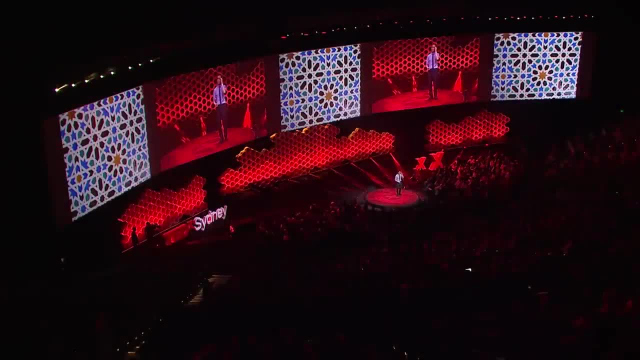 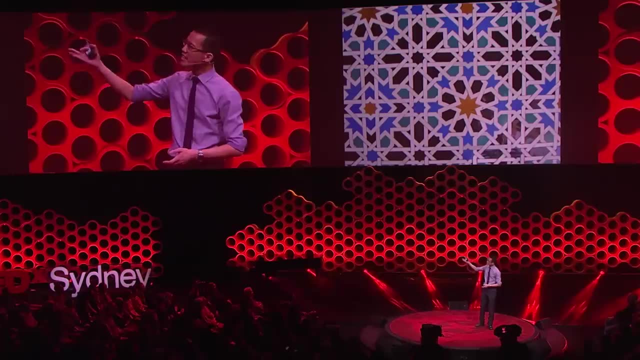 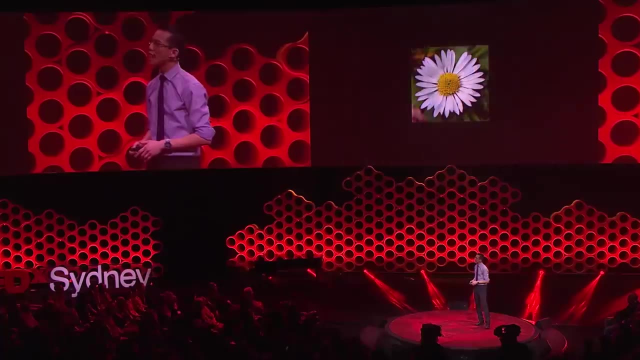 art and design. An aversion to depicting humans and animals led to a rich history of intricate time arrangements and geometric forms. The aesthetic side of mathematical patterns like these brings us back to nature itself. For instance, flowers are a universal symbol of beauty. Every culture around the planet. 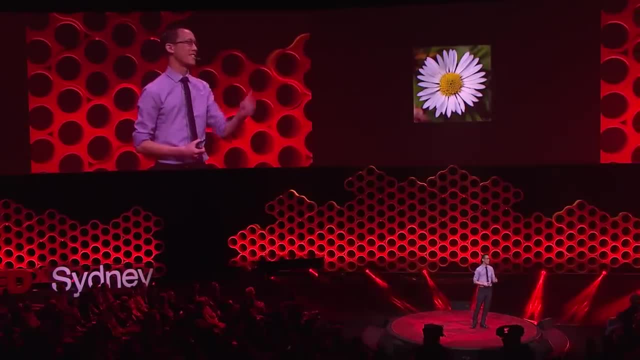 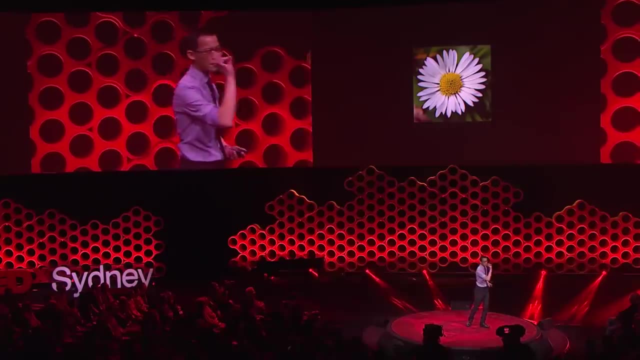 and throughout history has regarded them as objects of wonder. One aspect of their beauty is that they exhibit a special kind of symmetry. Flowers grow organically from a center that expands outwards in the shape of a spiral. Flowers grow from a center that expands outwards. 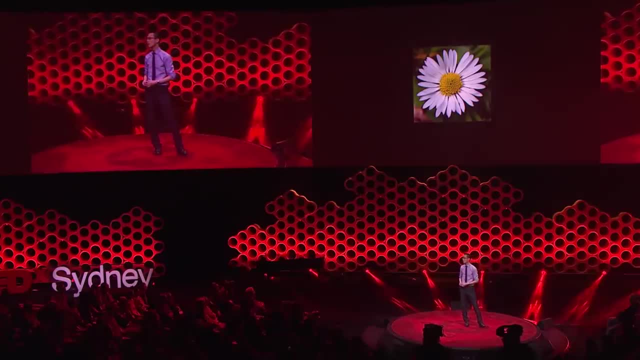 in the shape of a spiral. Flowers grow from a center that expands outwards in the shape of a spiral. Flowers grow from a center that expands outwards in the shape of a spiral. This creates what we call rotational symmetry. You can spin a flower around and around and